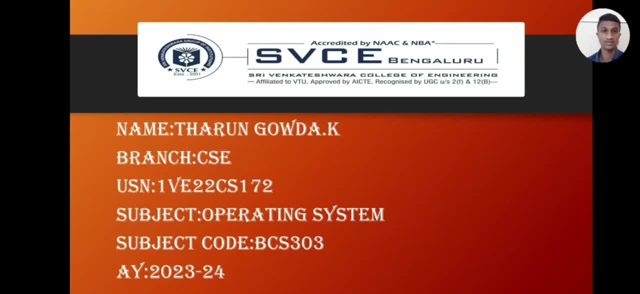 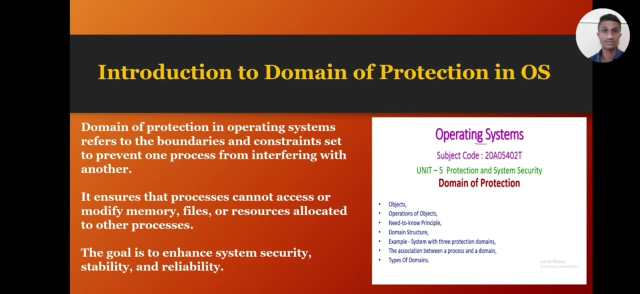 Hello everyone, myself Tarun from Sri Venkateshwara College of Engineering, 3rd semester, CSC department. Now let us discuss about a topic related to operating system that is, domain of protection. Introduction to domain of protection. Domain of protection in operating systems refers to the boundaries and constraints. 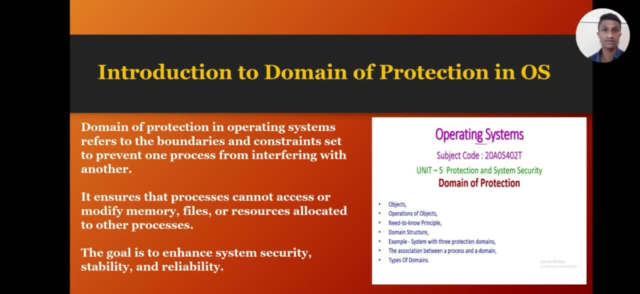 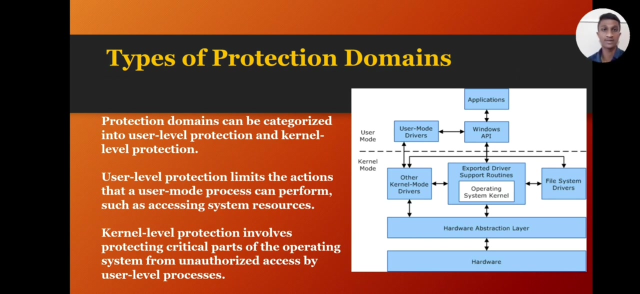 set to prevent one process from interfering with another. It ensures that processes cannot access or modify memory files or resources allocated to the other processes. The goal is to enhance system security, stability and reliability. Types of protection domains: Protection domains can be categorized into user-level protection and kernel-level protection. 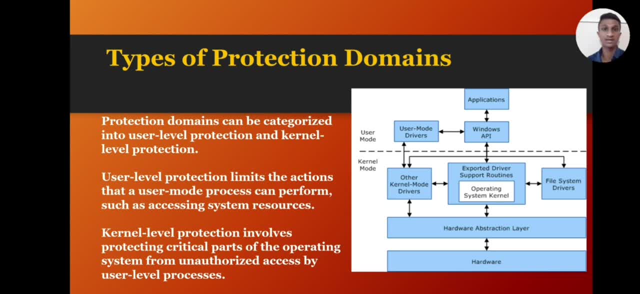 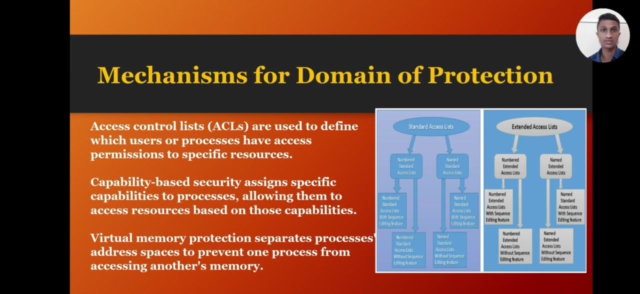 User-level protection limits the actions that occur The user-mode process can perform, such as accessing system resources. Kernel-level protection involves protecting critical parts of the operating system from unauthorized access by user-level processes. Mechanisms for domain of protection- Access control lists- are used to define which users or processes have access permissions to specific resources. 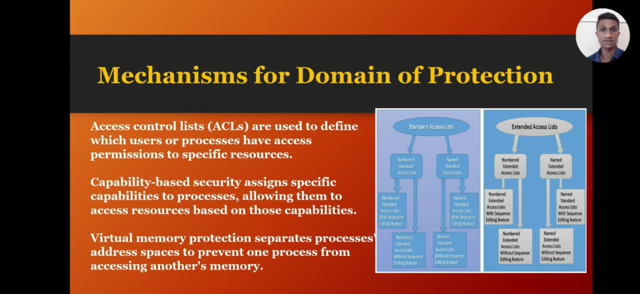 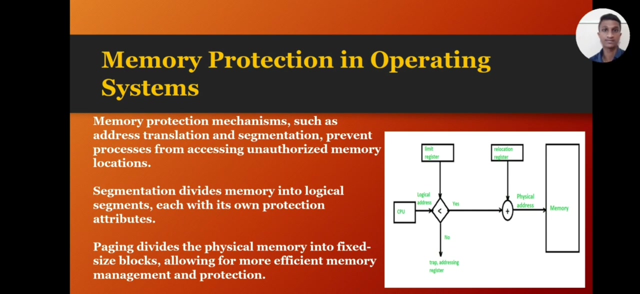 Capability-based protection Security assigns specific capabilities to processes, allowing them to access resources based on the capabilities. Virtual memory protection Separates processes' addresses spaces to prevent one process from accessing another's memory. Memory protection in operating system: Memory protection mechanisms such as address, translation and segmentation. 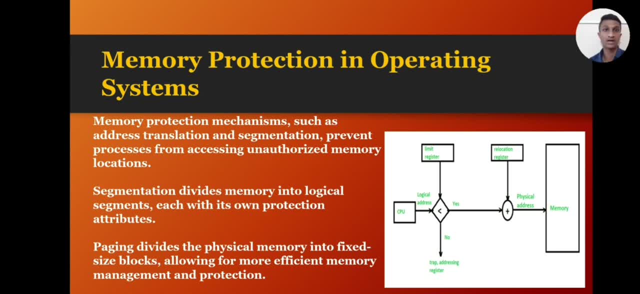 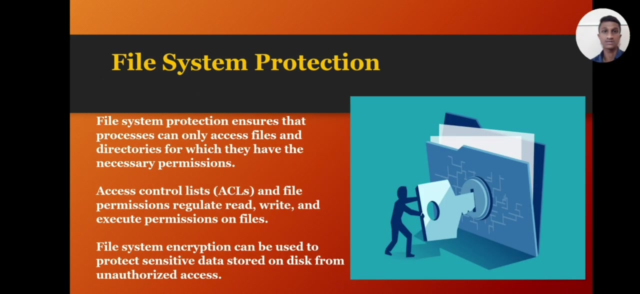 prevent processes from accessing unauthorized memory locations. Segmentation divides memory into logical segments, each with its own protection attributes. Paging divides the physical memory into fixed-sized blocks, allowing for more efficient memory management and protection. File System Protection. File system protection ensures that processes 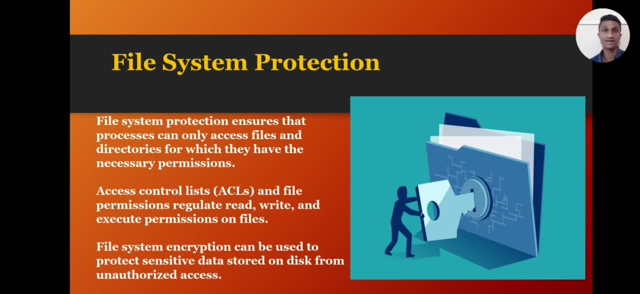 can only access files and directories for which they have the necessary permissions. Access control lists and file permissions. regulate read-write and execute permissions on file File system encryption can be used to protect sensitive data stored on disk from unauthorized access, Network Security and Domain Protection. 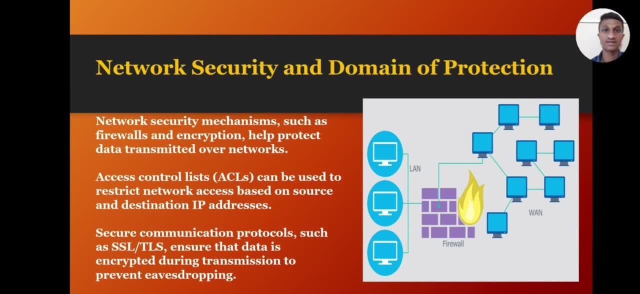 Network Security and Domain Protection. Network security mechanisms such as firewalls and encryption help protect data transmitted over networks. Access control list can be used to restrict network access based on source and destination IP addresses. Secure communication protocols such as SSLs and TLS ensure that data is encrypted during. 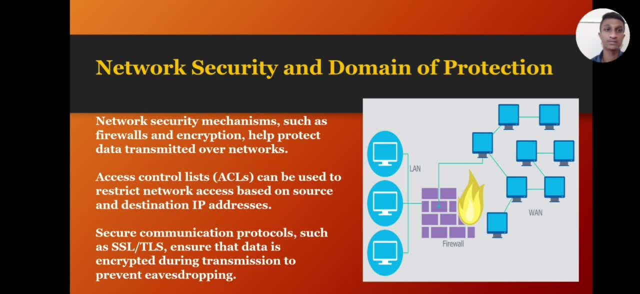 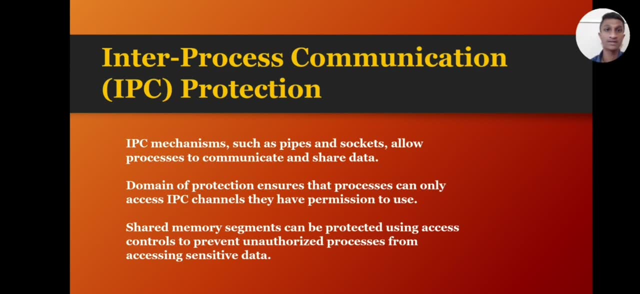 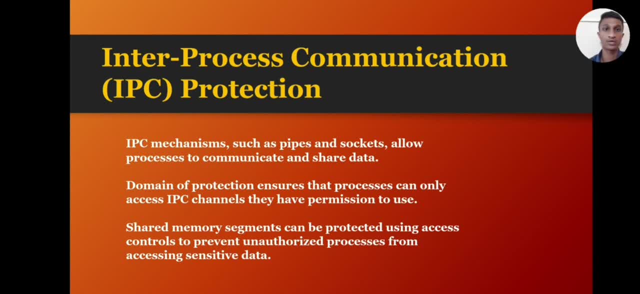 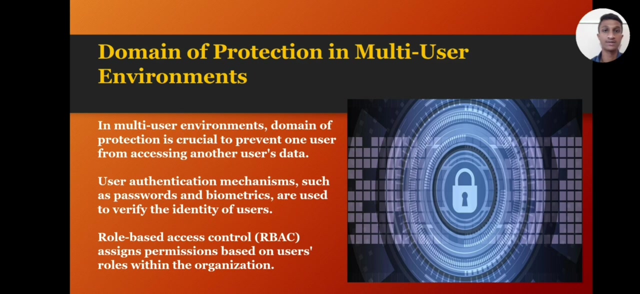 하 sharp conquest Musk Agent Chain processes from accessing sensitive data. domain of protection in multi-user environments. in multi-user environments, domain of protection is crucial to prevent one user from accessing another users data. user authentication mechanisms such as passwords and biometrics are used to verify the identity of users. role-based access control, RBAC- assigns permission based on. 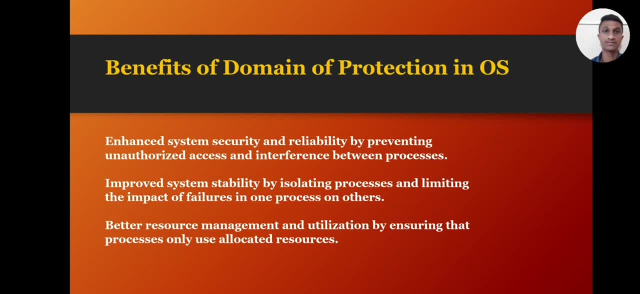 users role within the organization. benefits of domain of protection in operating system: enhance its system security and reliability by preventing unauthorized access and interference between processes. improved system stability by isolating processes from accessing data from other systems and limiting the impact of failures in one processes and others. better resource.